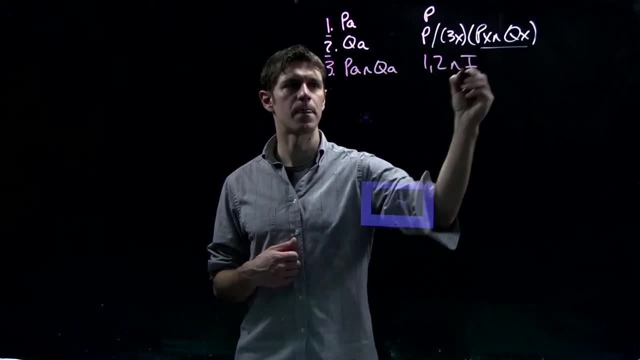 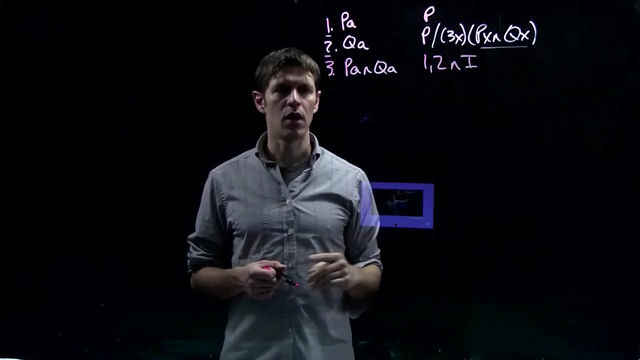 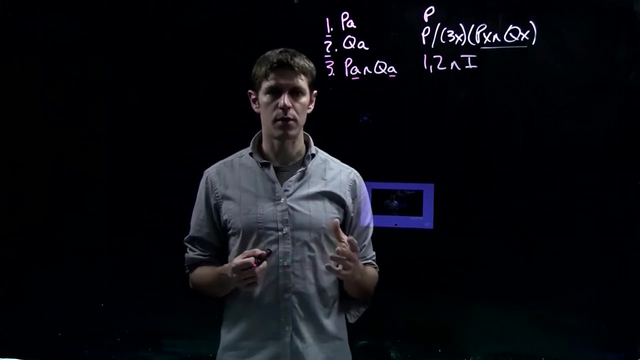 So this is by 1-2 conjunction introduction. But now that we have this conjunction we can make use of existential introduction. And in using existential introduction we can replace at least one of the names in this formula at line 3 with an existentially quantified variable. 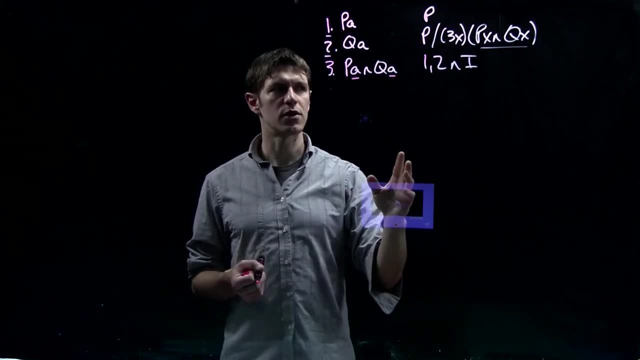 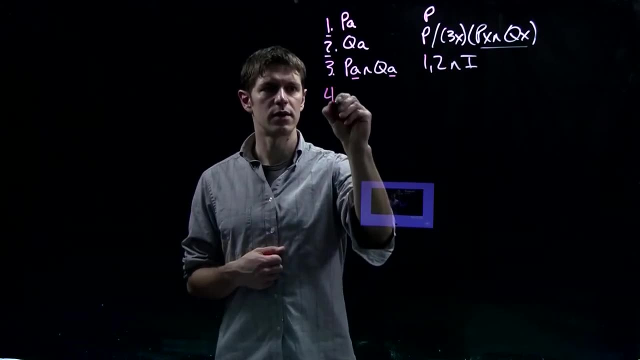 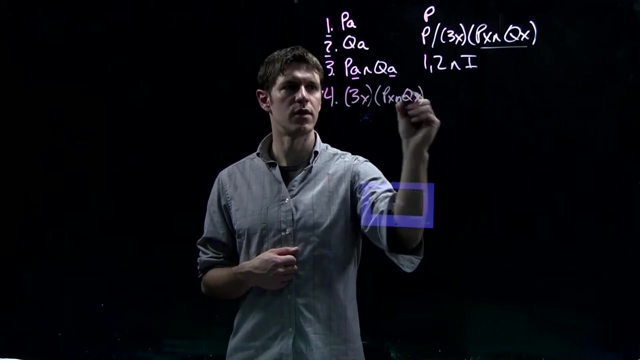 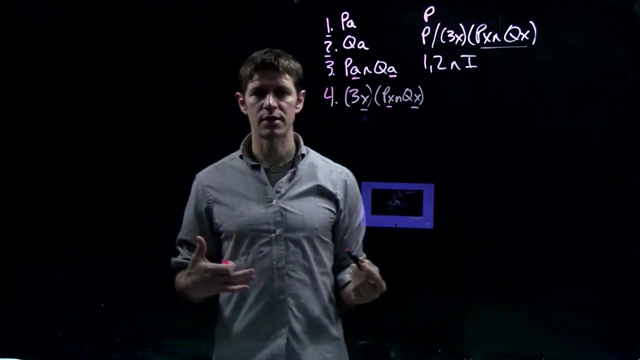 And if we replace more than one name, then we need to make sure the replacement is uniform. That is, we're replacing the same name with the variable, So we can write EX, PX and QX, So we're replacing. We're replacing these names A with the variable X, and this variable is quantified by the existential quantifier. 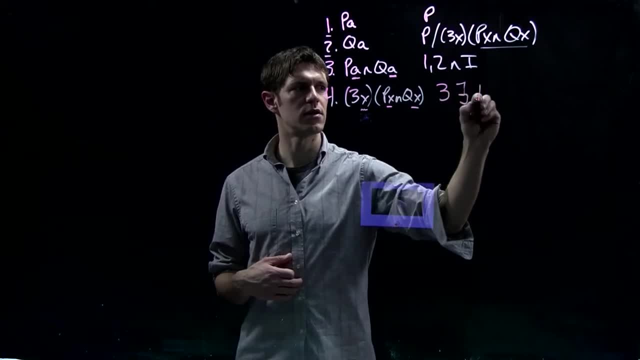 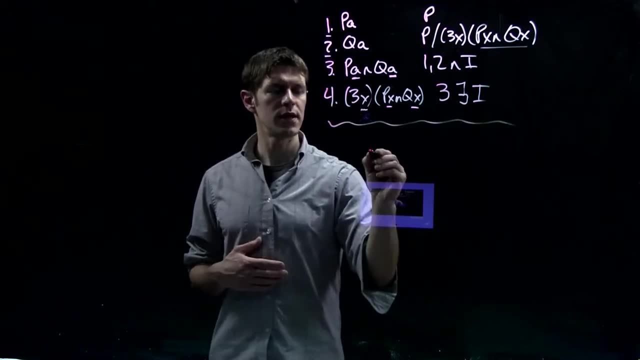 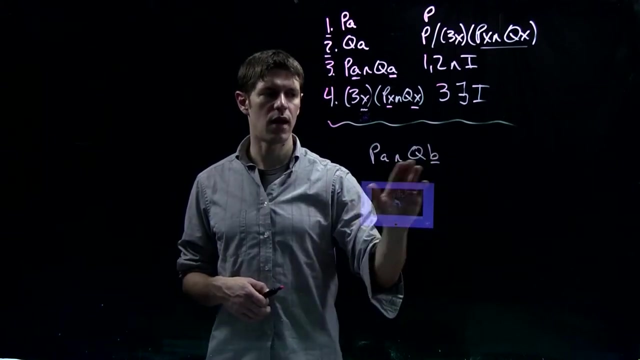 So this is from line 3, existential introduction. There's a couple things to note about this particular proof. Let's say we had PA and QB instead. So rather than having A and A, we have A and B, If we were to use existential introduction on this one. 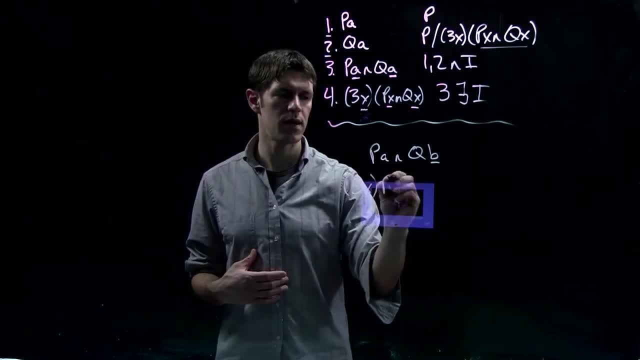 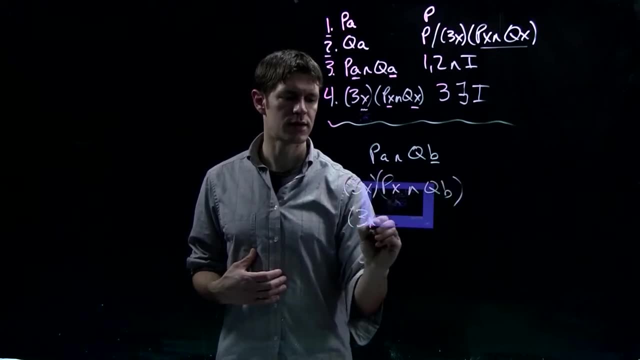 we would have A and B. If we were to use existential introduction on this one, we would have A and B. So in this formula we could reason to EX PX and QB, Or we could reason to EX PA and QX. 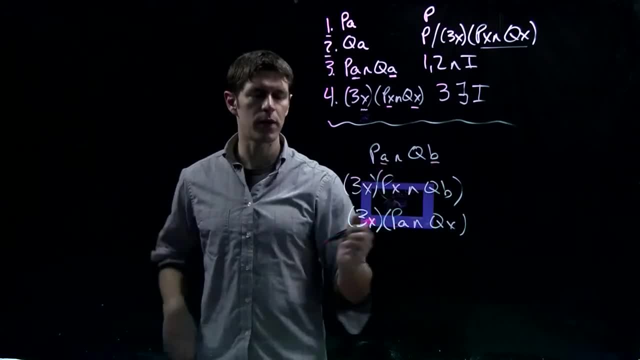 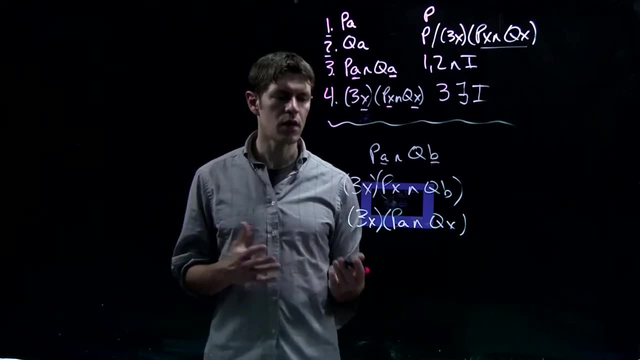 So, since this is not the same name, we can't replace both of the variables with a single existentially quantified variable. In addition, going back to 4, right here, another formula we can use is the one that we have in line 3.. 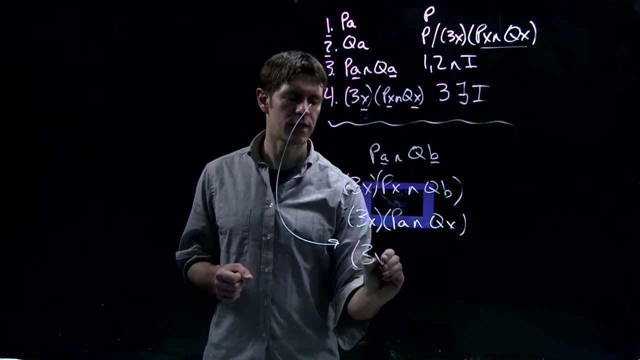 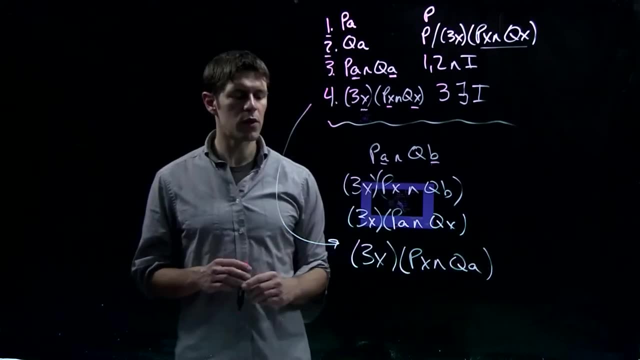 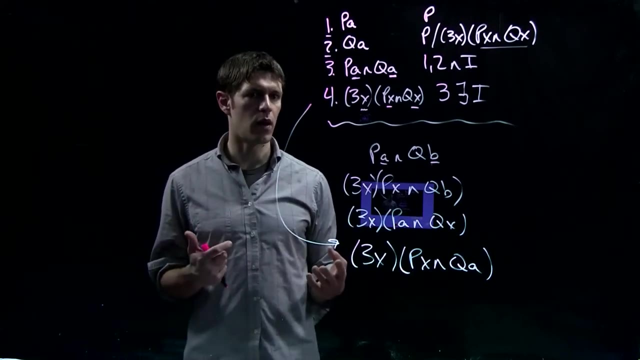 Another formula that we can reason to would be EX, PX and QA, So we're not required to replace all the names with an existentially quantified variable, but whenever we want to replace more than one, we need to make sure it's the same name with the same variable. 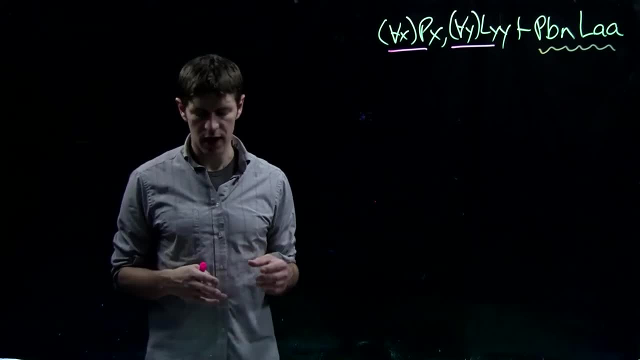 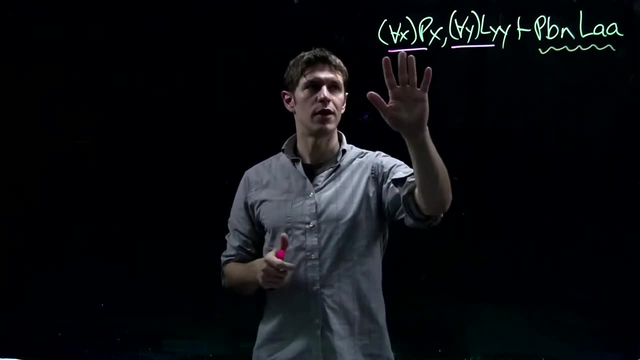 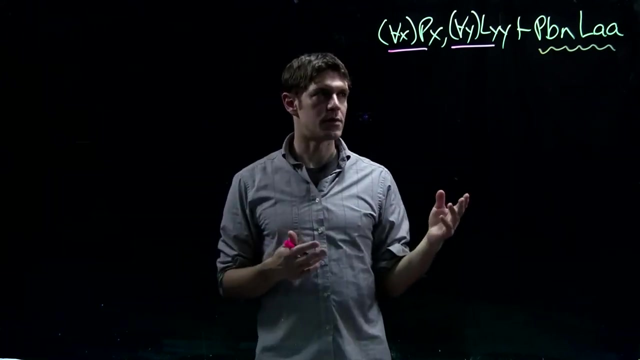 So let's look at a proof that focuses on the use of universal elimination. So here I have our example, our entailment set up here. We have AXPX, or everyone's a person, We have AYLYY, or everyone loves themselves. And then we want to reason to: let's say, Bob is a person and Al loves. 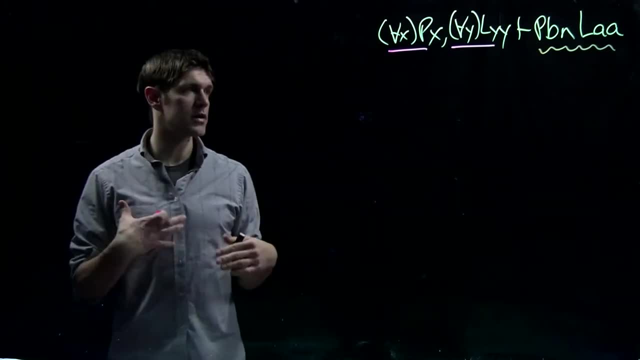 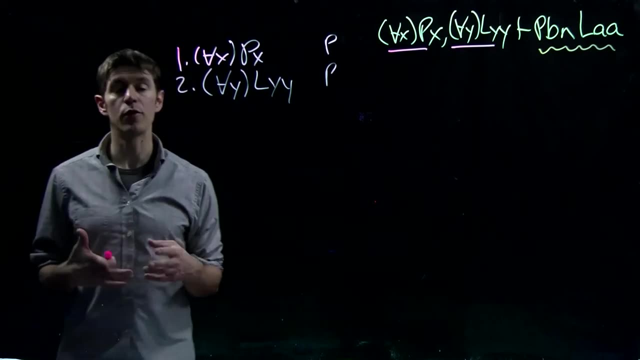 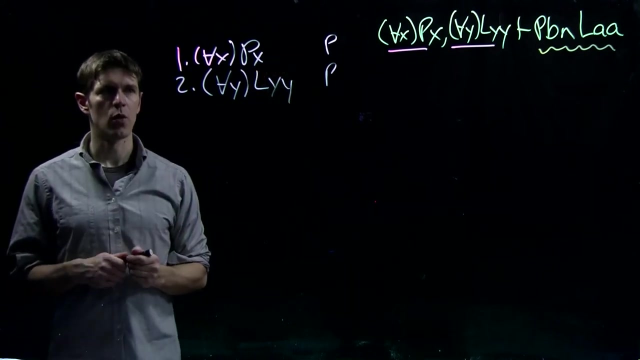 Al or Al loves himself. So we'll set the proof up by writing out the two formulas. So let's do that first. Now that we have the proof or derivation set up, the goal will be to reason to the conclusion. So we'll start by taking the first formula, which is AXPX, and reasoning to 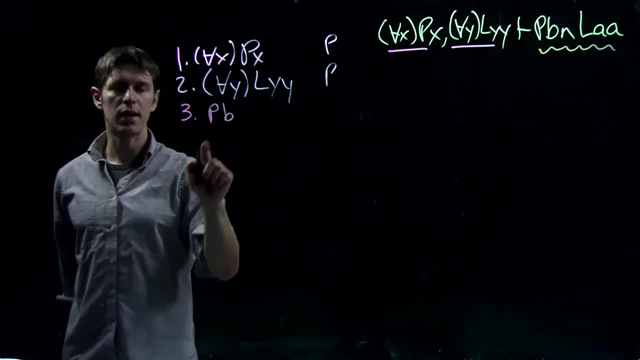 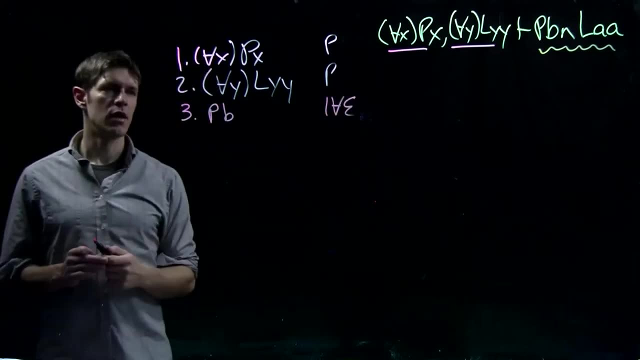 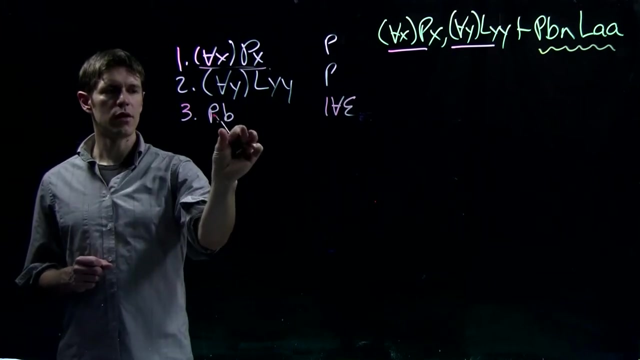 PB And the way we get PB, the way we derive PB, is by using line one and the universal elimination rule. The universal elimination rule allows us to reason from a universally quantified formula to an unquantified formula or to a formula where we're removing the universal. 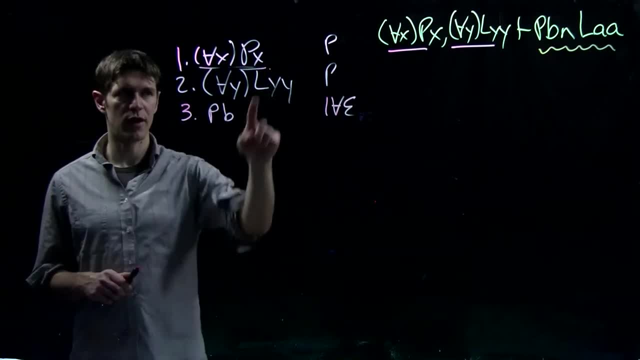 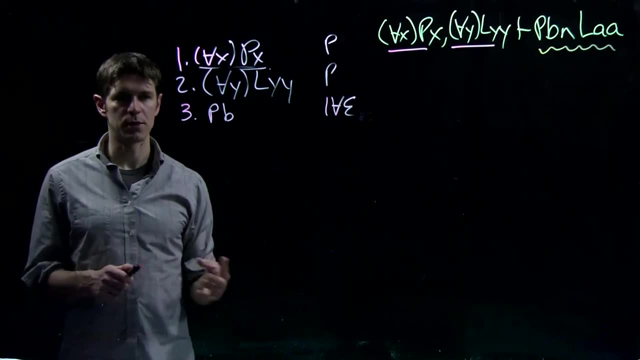 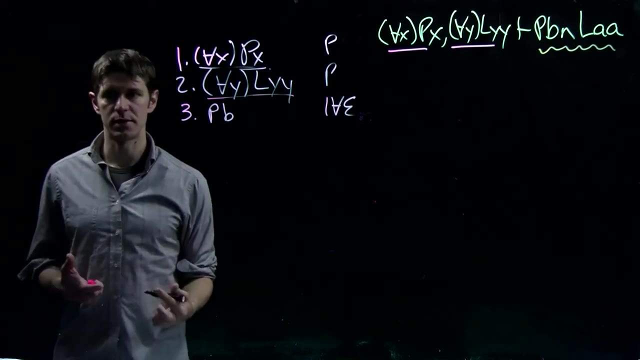 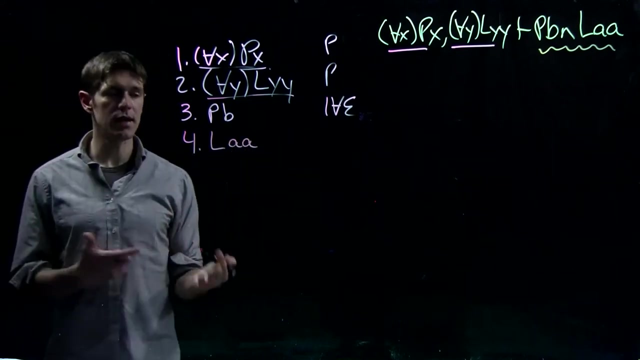 quantifier And replacing every bound variable X, every universally quantified variable that's bound with any name that we want And the replacement again must be uniform. So now that we have PB, we can use line two, which says everyone loves themselves to reason, to LAA- We could pick any. 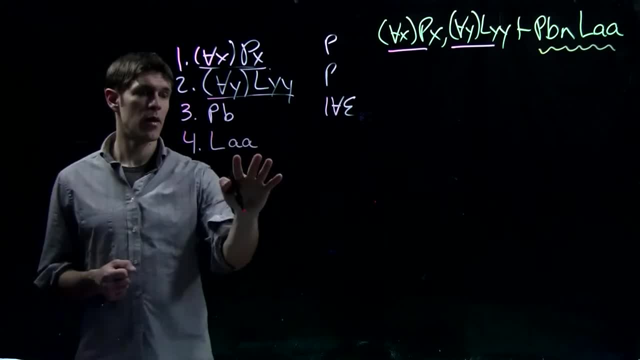 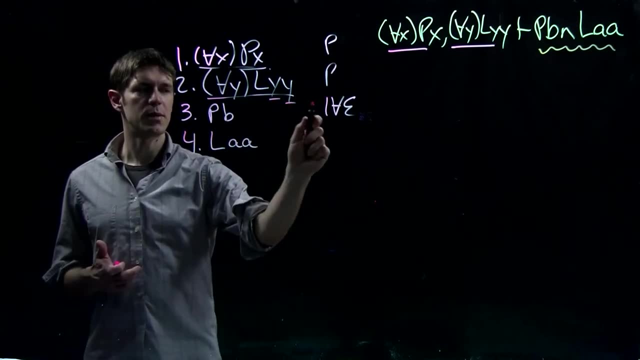 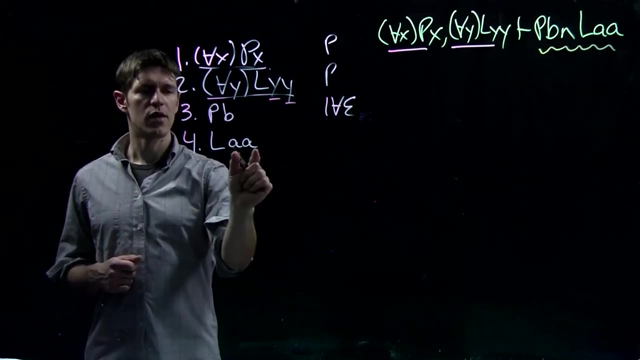 name that we wanted BB or CC or DD. but the reason we and the reason we pick here A here is because it's in the conclusion And we also need to note that the replacement must be uniform. So if we are going to replace these two universally quantified variables Y, then we need to make 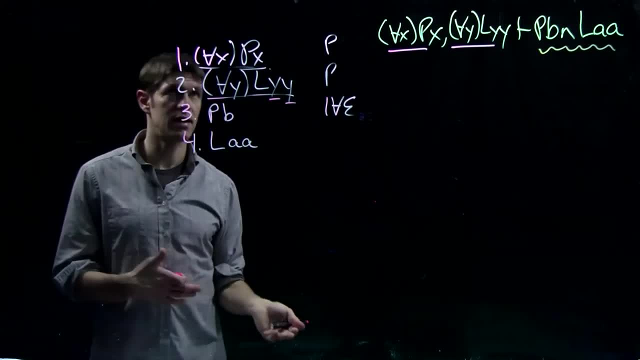 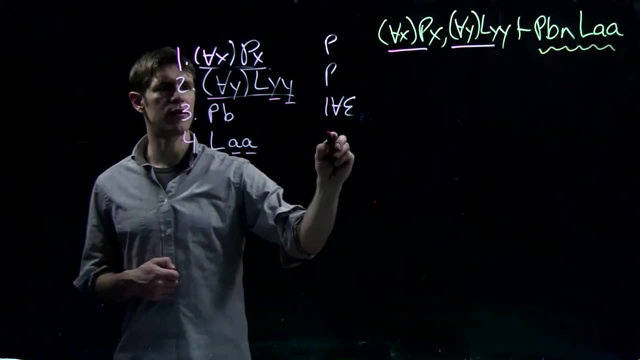 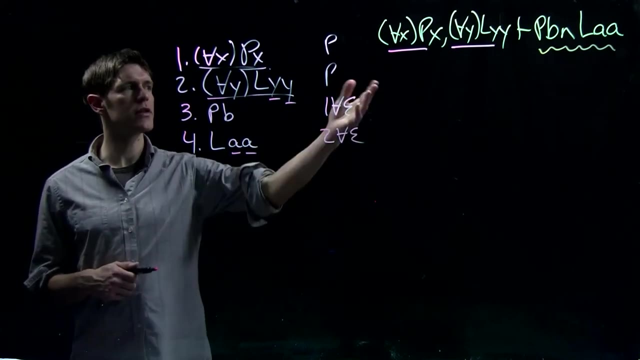 sure it's BBCC, not AB, not BC, not a different combination. They need to be the same name. And so we have line two and we're reasoning to line four, And this is by two universal elimination. Now that we have these two formulas, we have 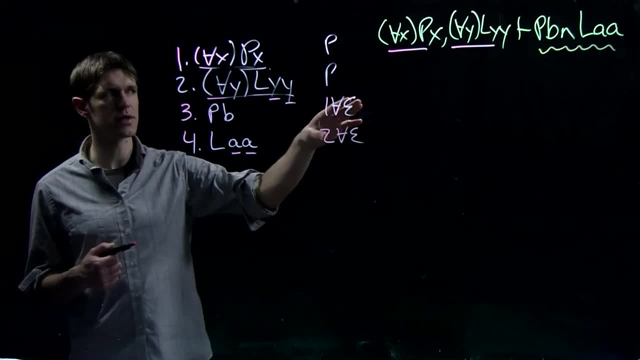 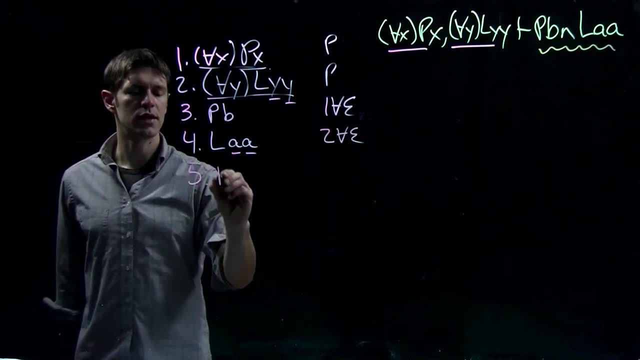 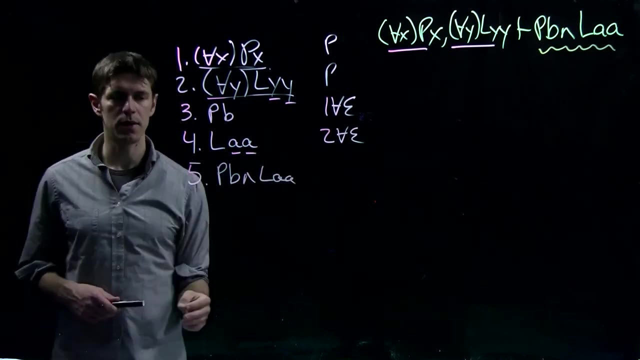 two ingredients or two formulas that are part of our conjunction, which is in the conclusion. We can take line three and line four and put those two formulas together using conjunction introduction, And so what I'm doing here is taking line three, which is PB line four. 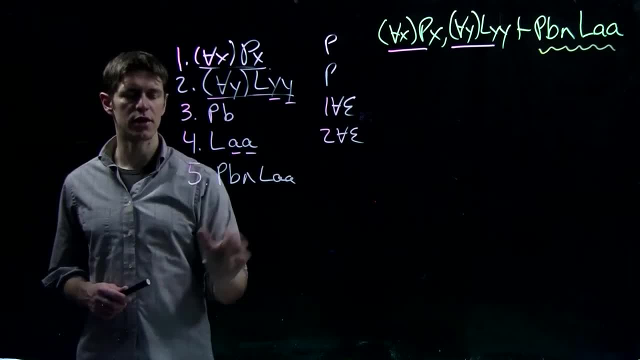 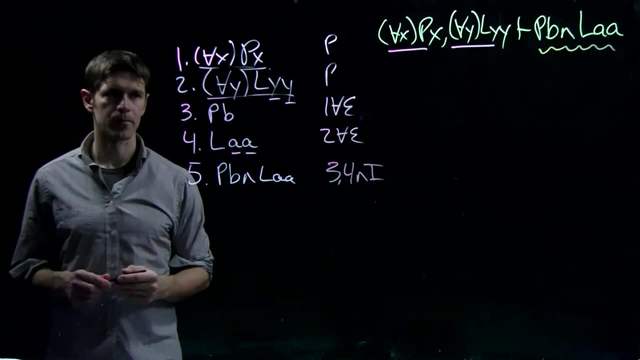 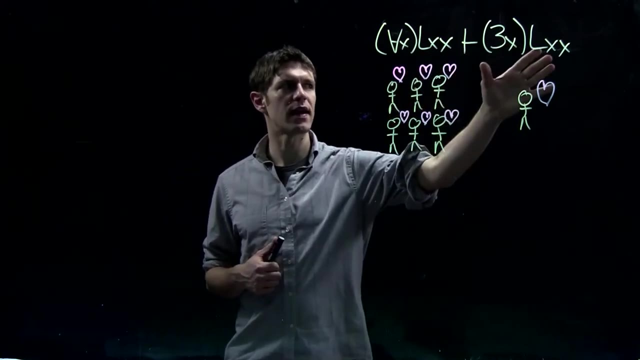 which is LAA, and reasoning to the conjunction of those two formulas. This is three for conjunction introduction. In the next proof we'll reason from AXLXX to EXLXX, that is, from the formula that everyone loves themselves to the formula that. 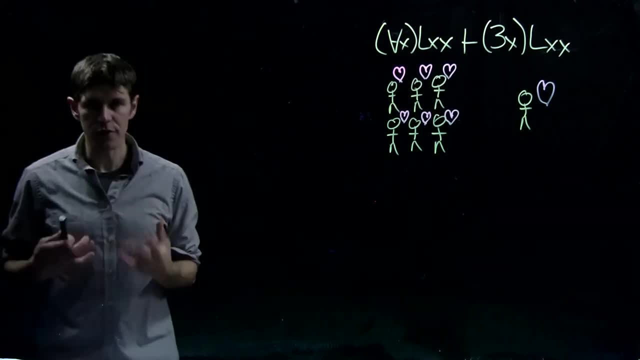 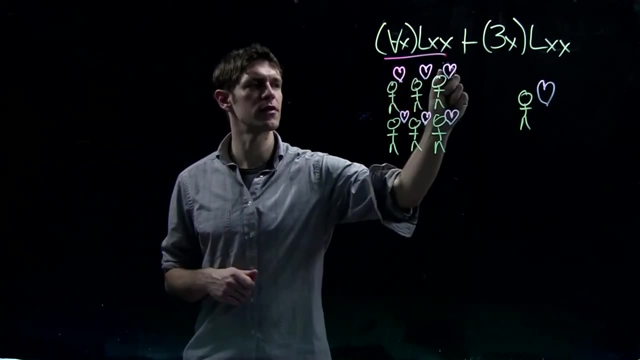 someone loves themselves. The first step in this proof is to set the whole thing up, and so we'll set it up by writing the formula to the left of the turnstile, and then we'll try to reason to the formula to the right of the turnstile. 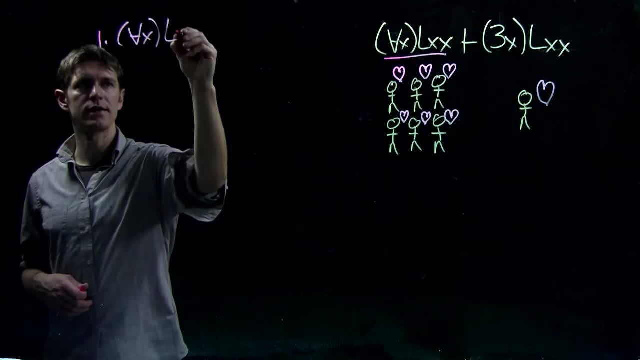 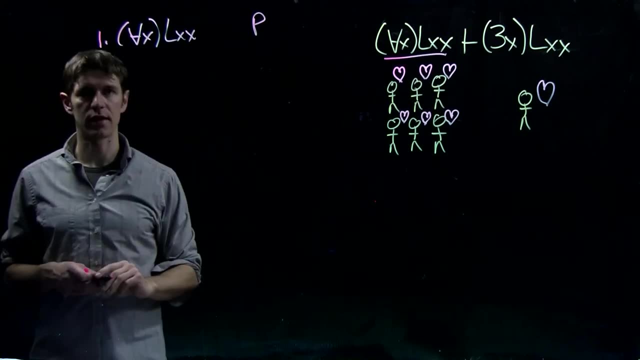 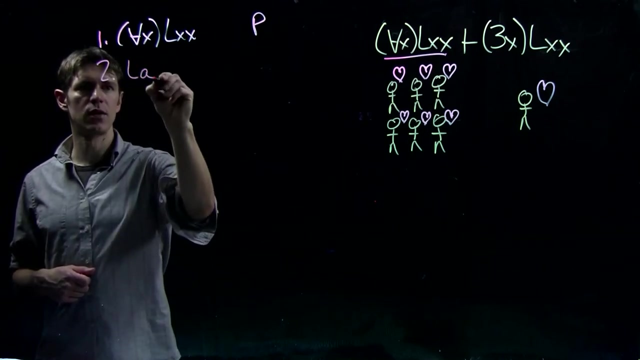 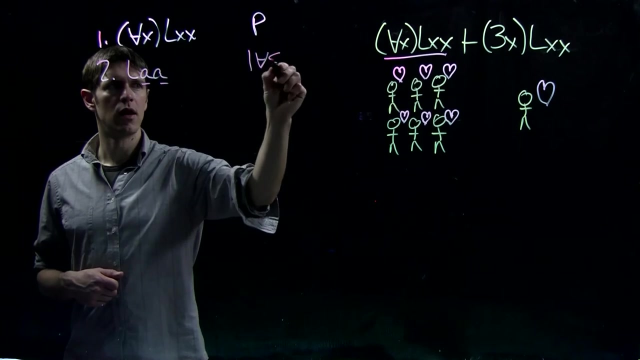 So we'll write LXX as a premise, and now the goal will be to reason to EXLXX. We'll start by using universal elimination and we'll replace each X with any name of our choosing, and here I'll pick A, and this is by one universal elimination. Now we can make use of existential elimination. 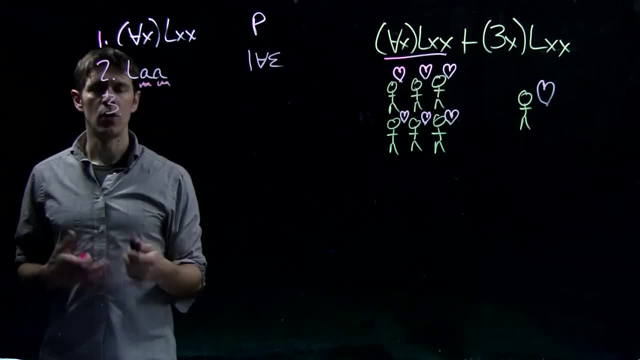 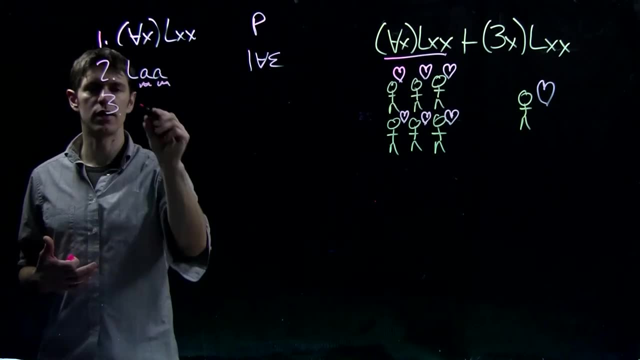 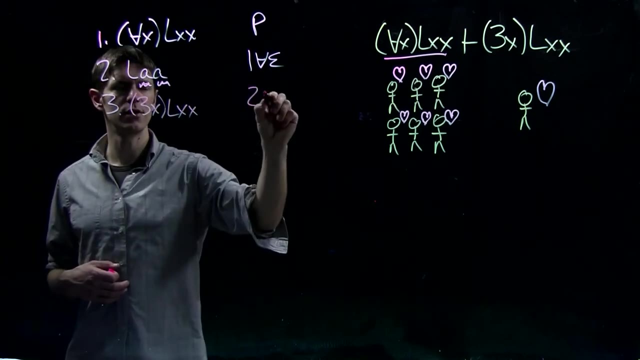 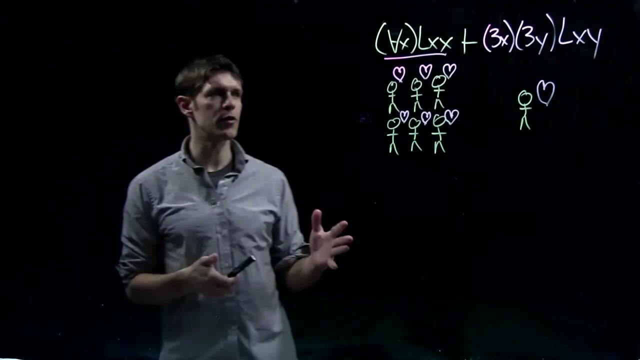 replacing each one of these A's with any name. replacing each one of these A's with the existentially quantified variable X, EXLXX, and this is, by line two, existential introduction. In this proof, we're reasoning from AXLX, that is, everyone loves themselves to the 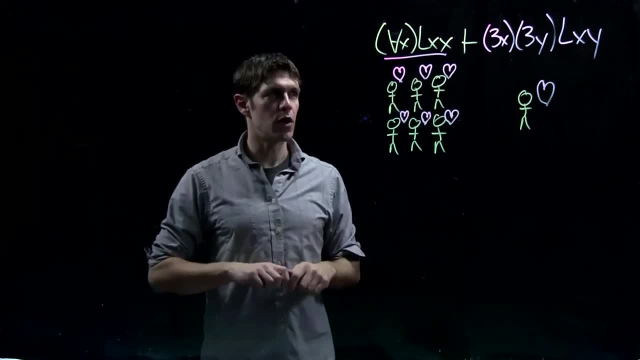 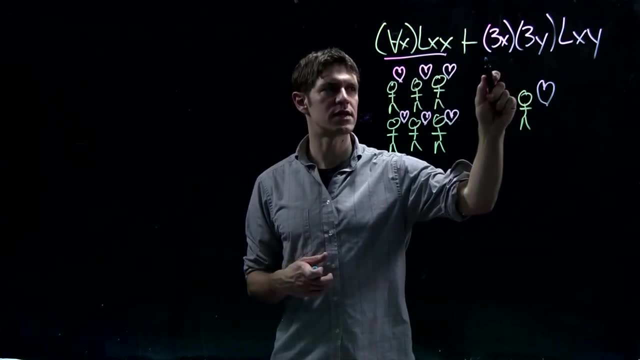 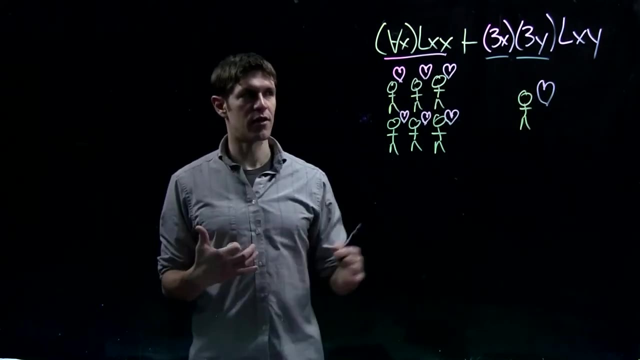 formula AXLX. It's important to note about this conclusion that this sentence does not say that is. this formula does not say that an individual loves another individual in the sense that this other individual is distinct from the first individual. It would be true, provided you have at least one individual. 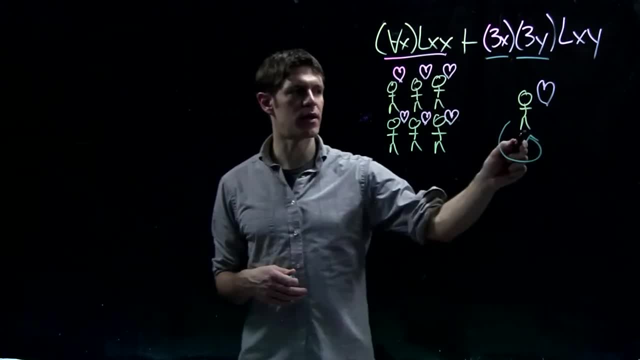 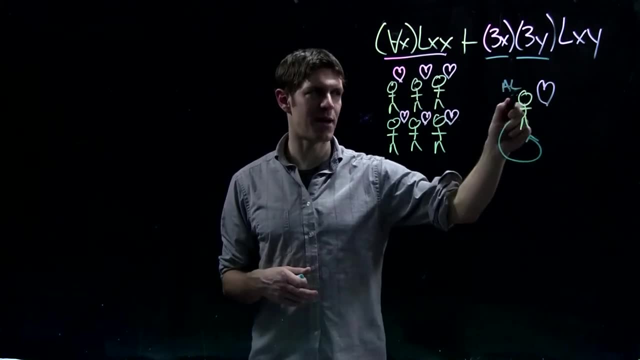 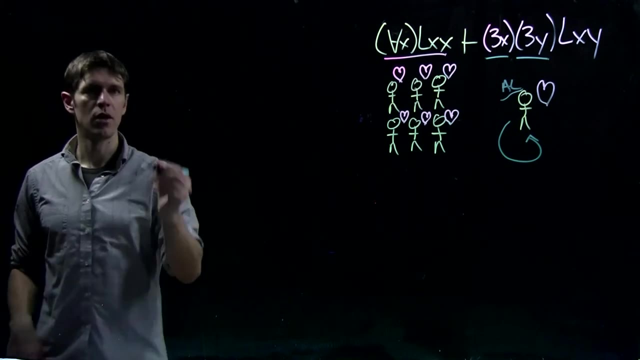 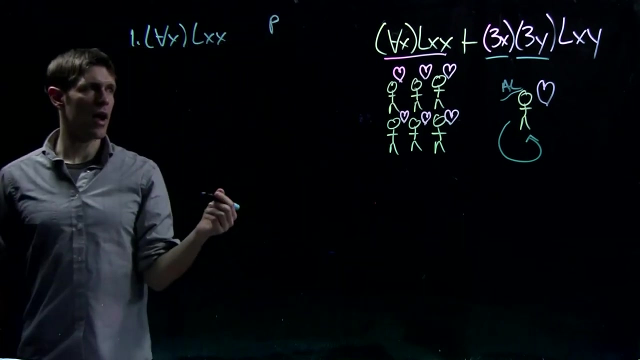 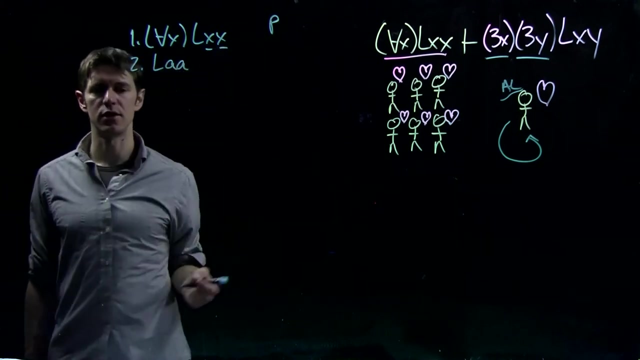 that loves themselves, because that's one individual- let's just call them L- who loves themselves. So we'll reason to or derive the conclusion from AXLXX. We'll start by setting up the proof, which is AXLXX, and we will next reason to LAA. We're replacing each one of these. 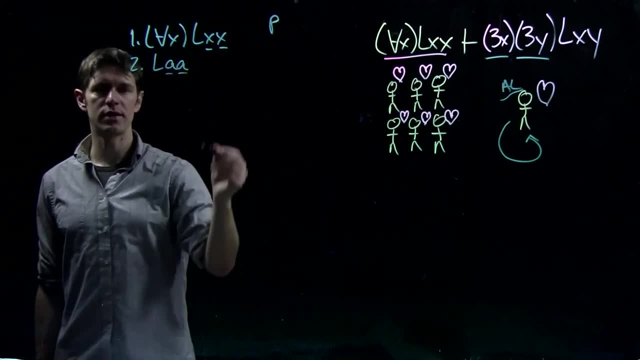 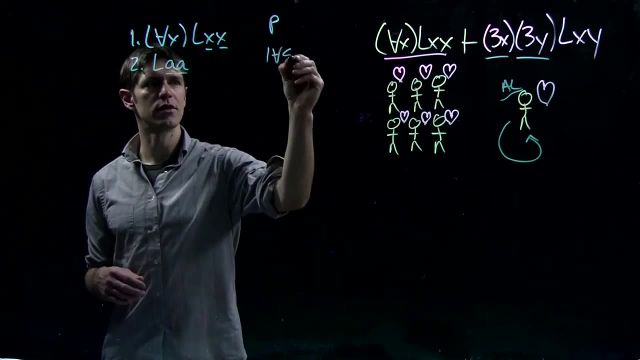 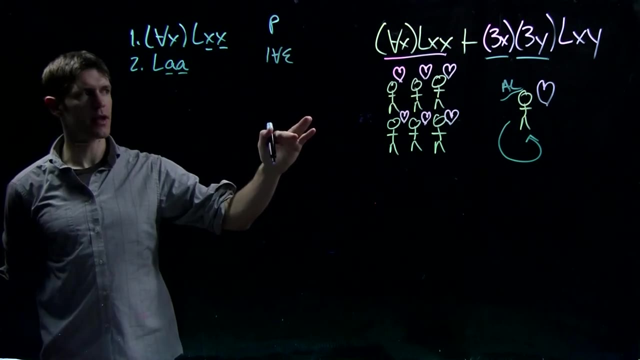 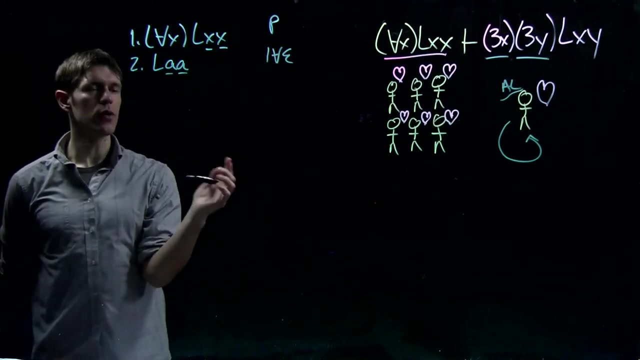 universally quantified variables with any name that we want, and we're making sure our replacement of these variables is with the same name, and this is by universal elimination. Now, in looking at our formula, which is the conclusion, we'll notice that we want to add two existential quantifiers here, and when we use existential introduction, we're only required to. 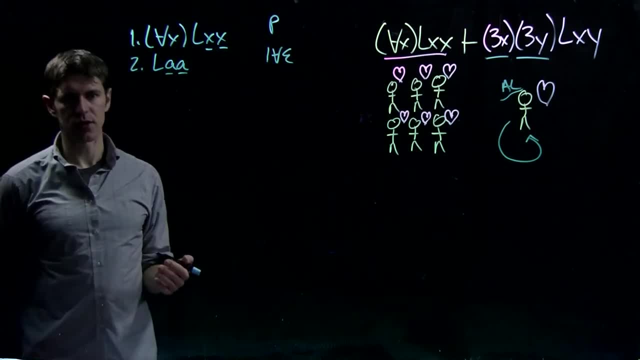 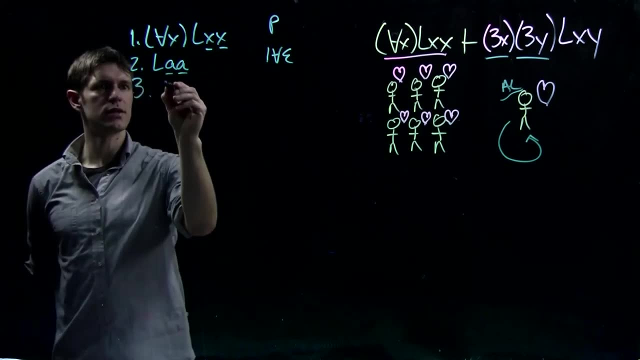 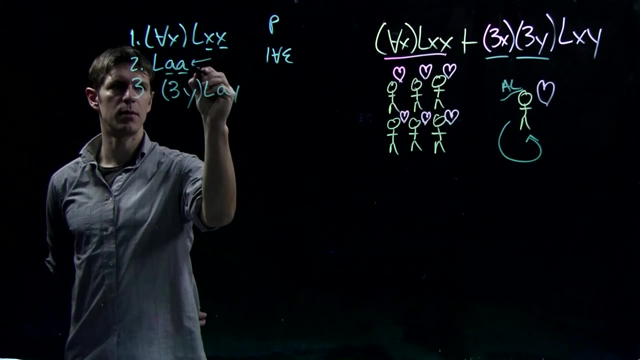 replace one of the names and replace it with an existentially quantified variable. We're not required to replace both of the names, and so at line three we'll reason to EYLAY. So we're replacing just this second name here with the existentially 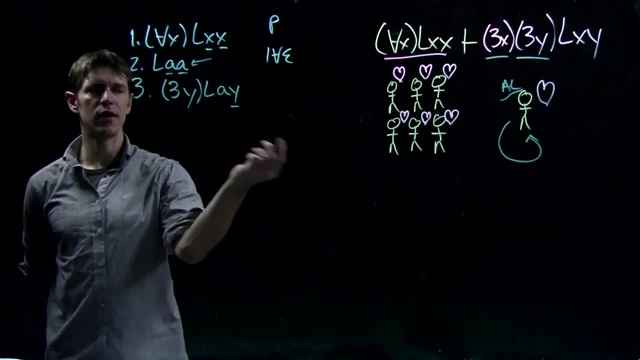 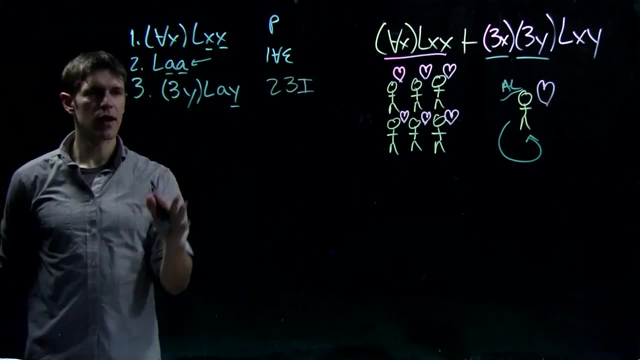 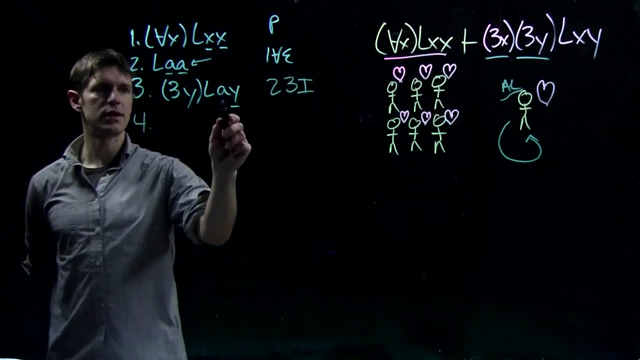 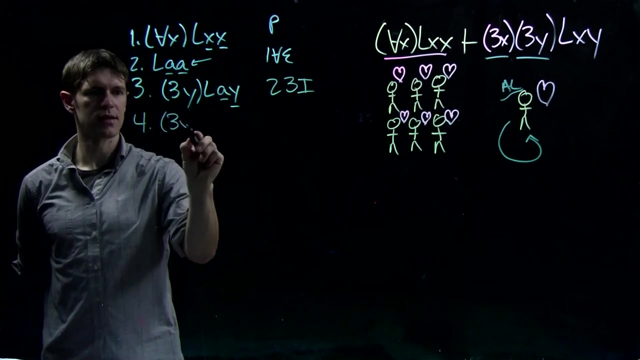 quantified variable Y, and so this says something like I'll love someone. and so this is, by line two, existential introduction. Now that we have this existentially quantified formula, at line three, we can use existential introduction on this formula, replacing this A with an existentially quantified variable, and so we can reason to EX. 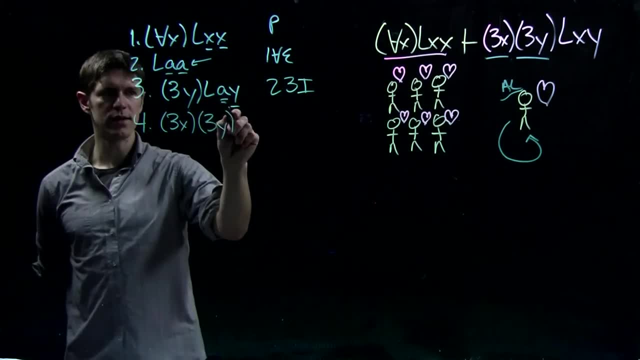 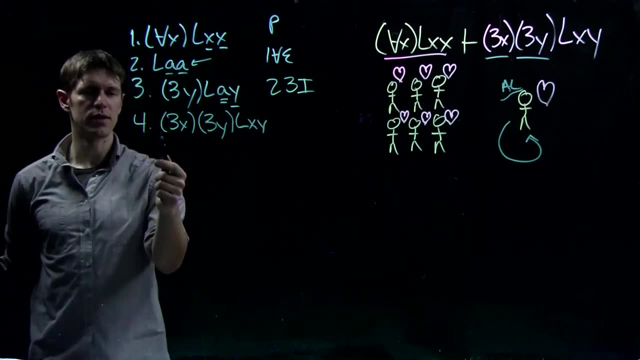 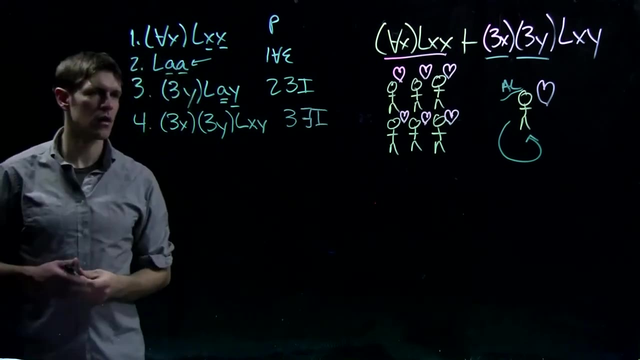 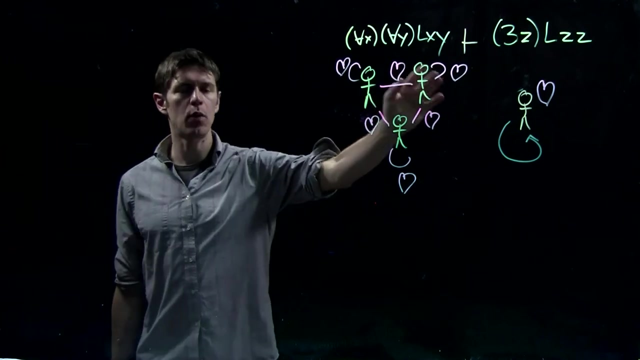 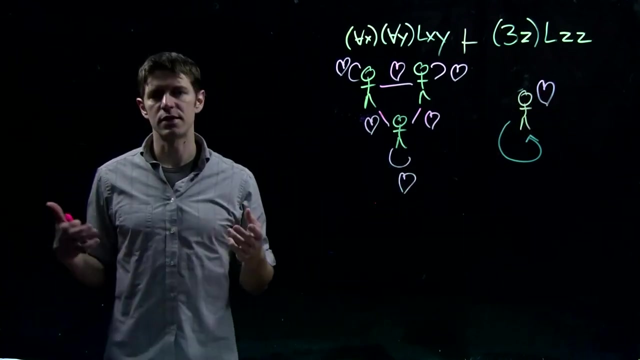 EY. and here we're replacing this A with an X, so it'll be LXY. and so from line three we reason to line four, using line three, existential introduction. In this proof, what we have is the quantified formula A-X-A-Y-L-X-Y and the conclusion is E-Z-L-Z-Z. To think about this in terms of an 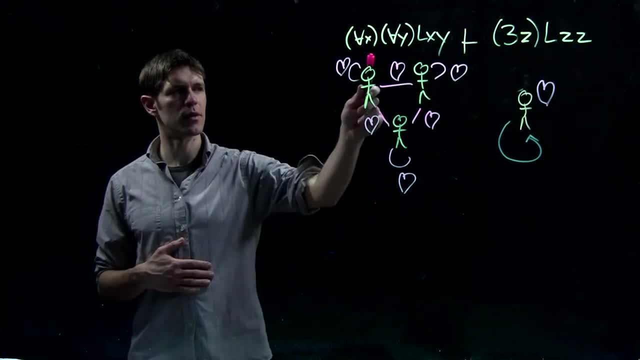 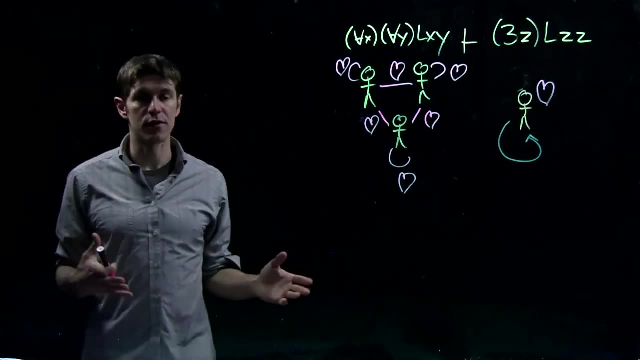 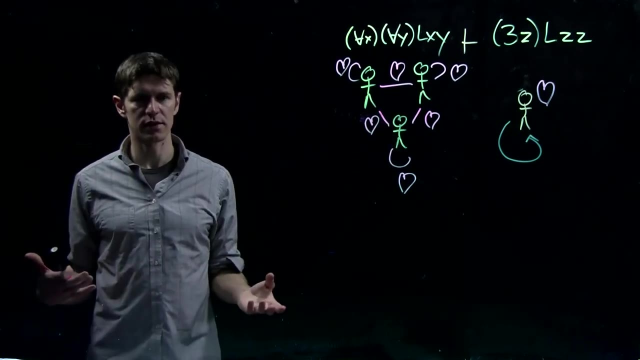 English argument. we might say that this particular formula says that everyone loves everyone, And we might think of a concrete example of this by imagining a domain of three people and each one of those individuals is in this loving relationship to everyone else in the domain. 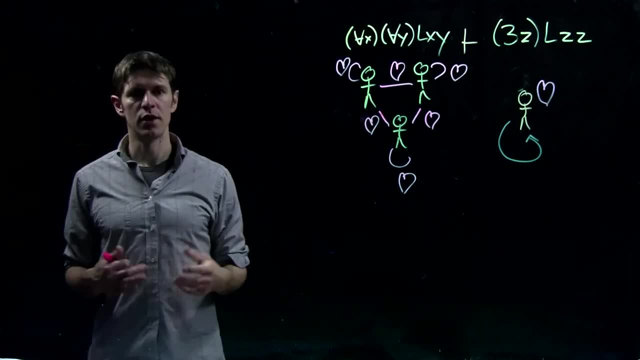 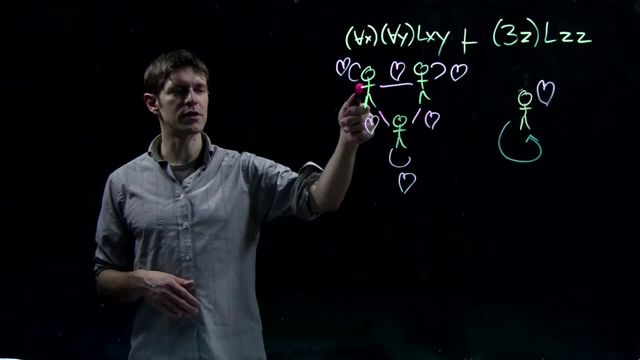 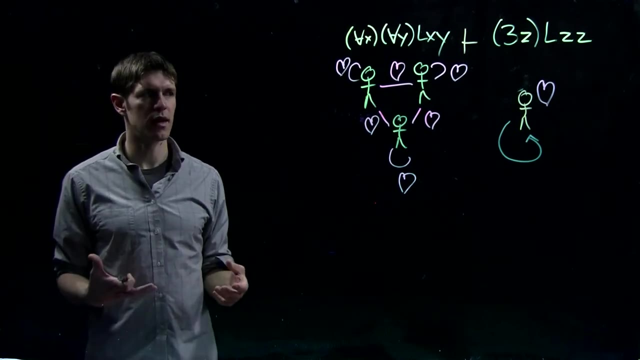 including in being a loving relationship to oneself. So not only does let's say Al love Liz and Liz love Tech and Tech love Al, but also Al loves Al, Liz loves Liz and Tech loves Tech. So every individual in the domain loves themselves, as well as everyone else in the domain We want. 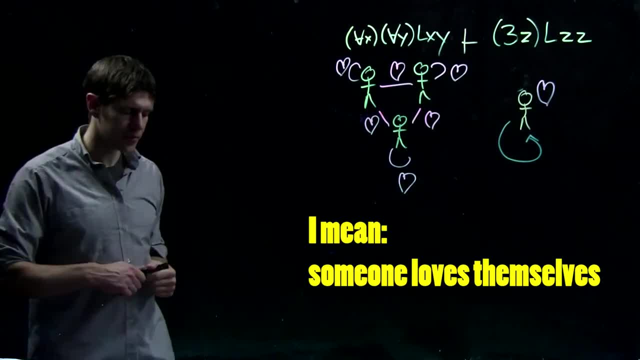 to reason, to the conclusion that someone loves someone. We'll start this proof by simply setting up the proof and thinking about it. So let's start this proof by simply setting up the proof and thinking about it. We'll start this proof by simply setting up the proof and thinking about. 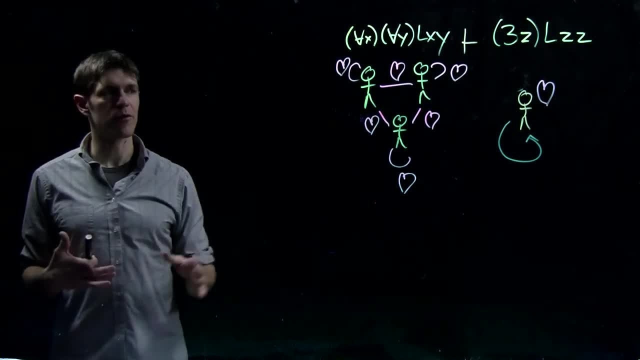 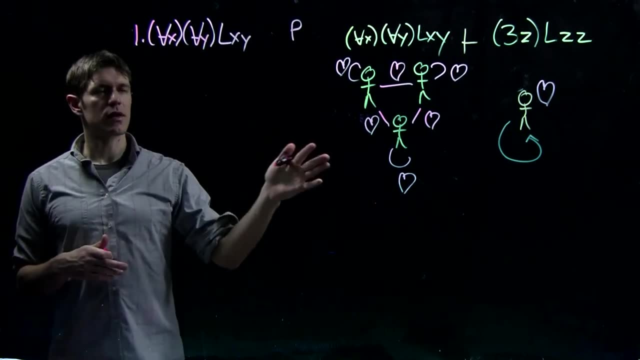 it. So let's start this proof by simply setting up the proof and thinking about it And since we have only one formula, we'll start the proof by simply writing this particular formula at line one. Now that we have this formula at line one, we'll reason to the conclusion And the way we'll go. 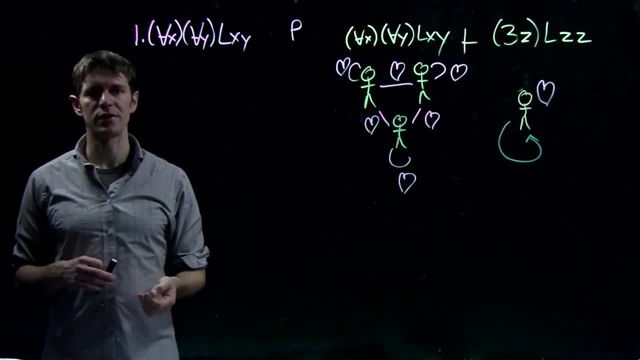 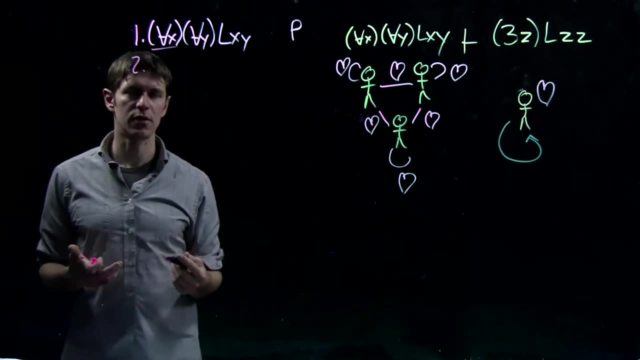 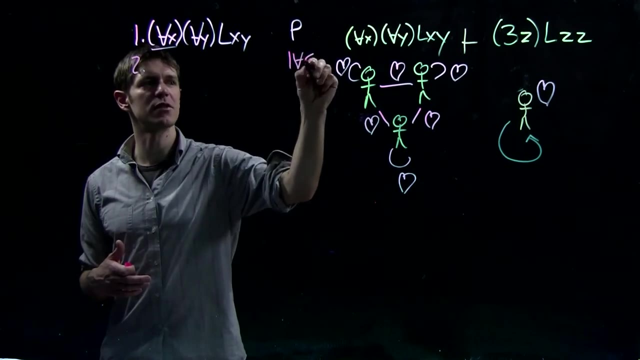 about doing this is by removing these universal quantifiers, using universal elimination. We'll start by removing the universal existential, removing, excuse me, the universal quantifier that binds for x, And so we'll use one universal elimination And we're removing this outermost quantifier. here We're removing the. 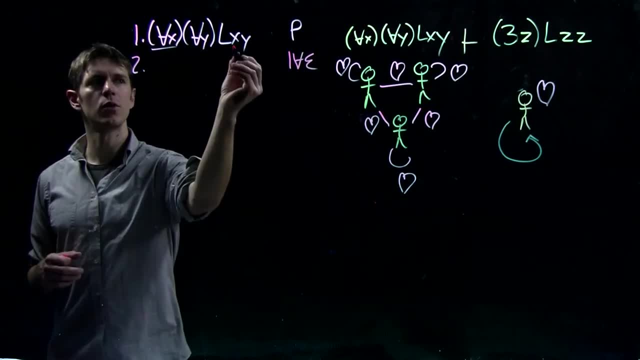 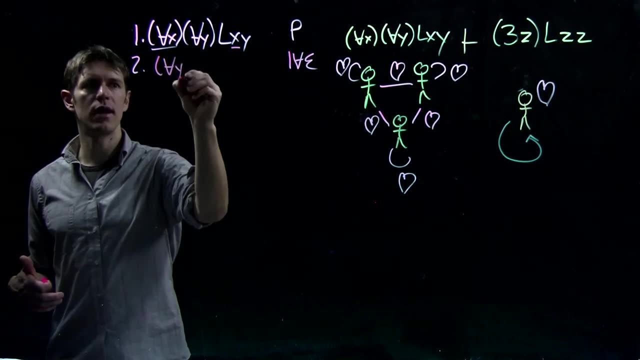 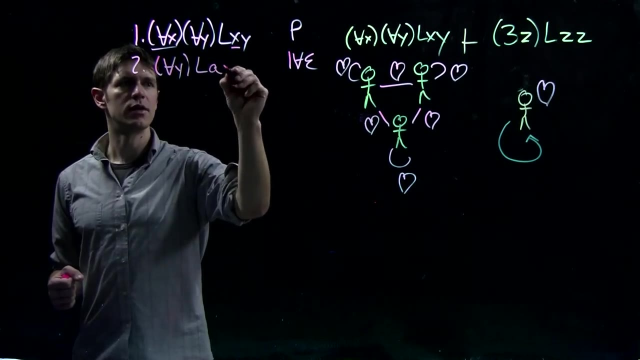 universal quantifier that's binding this x, And so we'll need to replace every instance of x with any name that we want, And so I'll write ay, here And now I want to make sure I replace this x with a name, And here I'm going to pick a, And so I'll leave the y alone. Now that I have this universally. 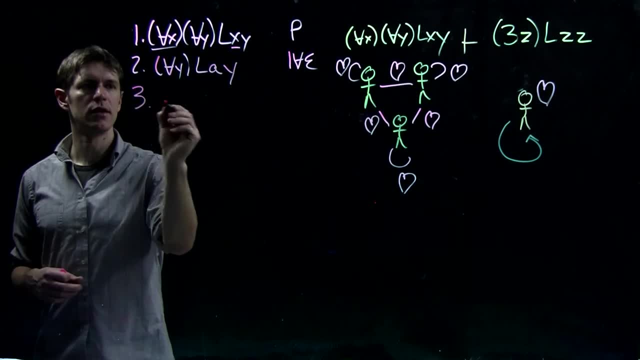 quantified expression at line two. I can now go ahead and use two more definitions, And so it's a little bit easier to go back to the original definition of the word evolution. but I'm going to, I'm going to reason using universal elimination again to a formula, And I want to make sure I 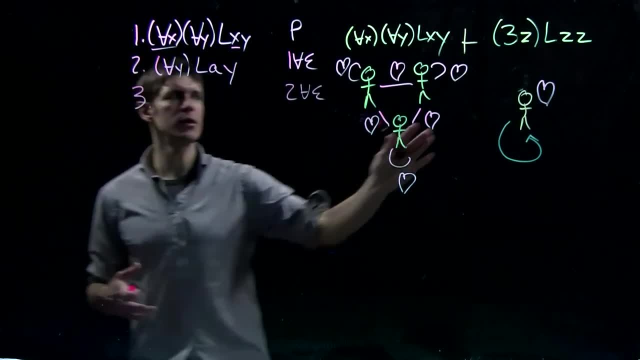 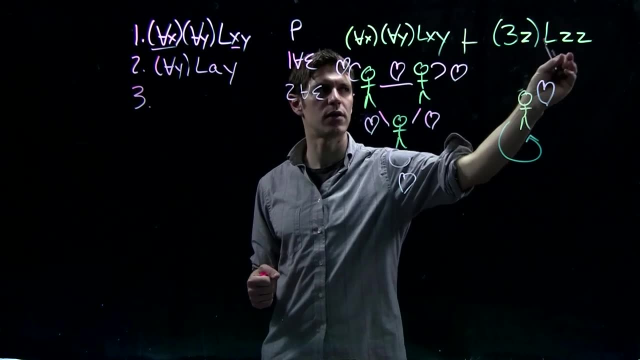 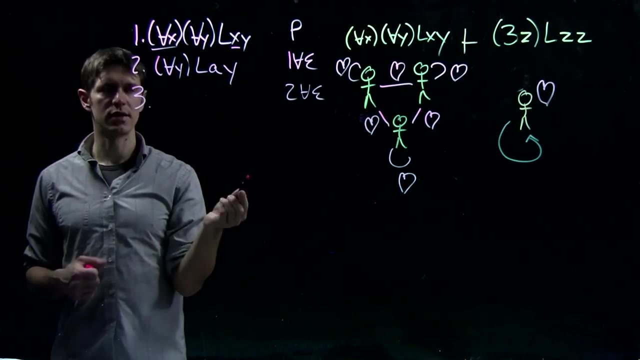 replace this y not with b. but since I ultimately want to make use of existential introduction here, replacing each of the names with an existentially quantified variable- and I want it to be the same variable, I will replace this y here with the name that I've already used, which is a. So I'll reason. 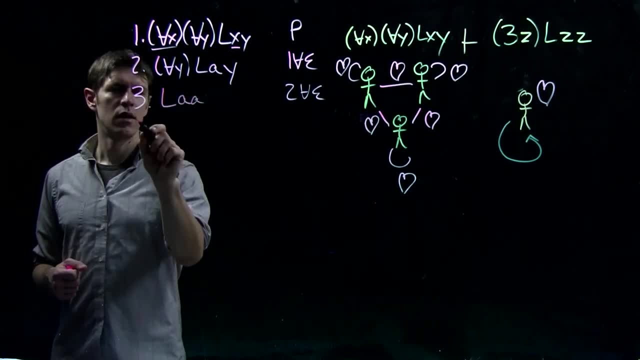 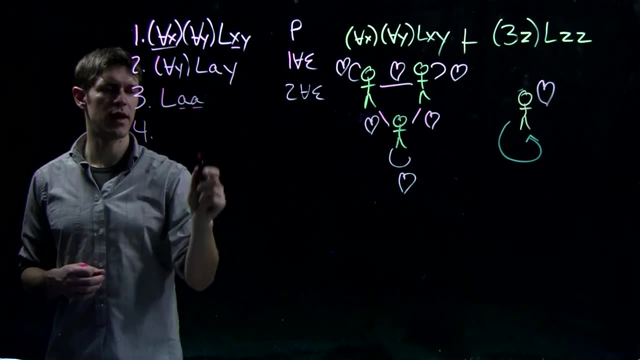 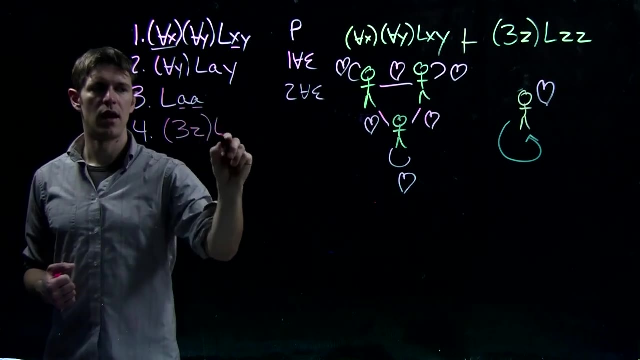 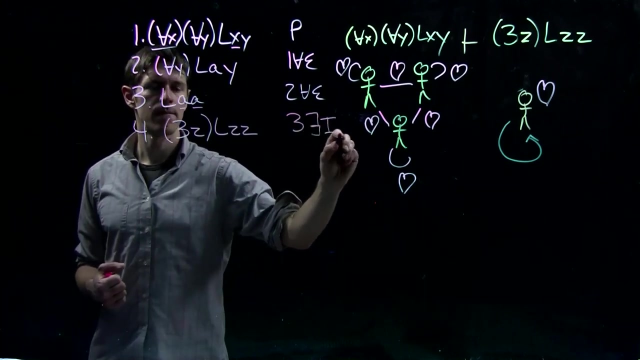 to al loves, al. Now, at line four, I can use the existential introduction rule, which allows me to take each one of these names and replace it with an existentially quantified variable. So I'll write e, z, l, z, z, And so this is, by line three, existential introduction. So what I've done here. 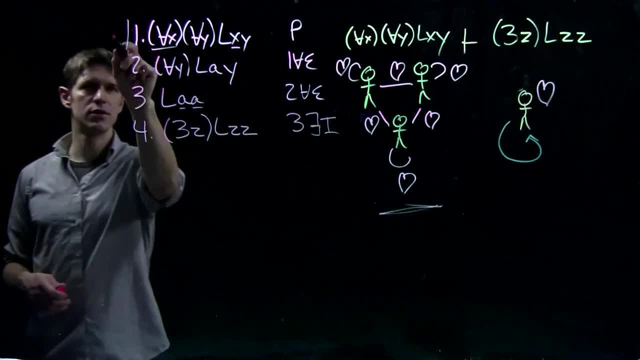 is reason from everyone loves everyone. this kind of state here two the sentence someone loves themselves, which is this state over here.